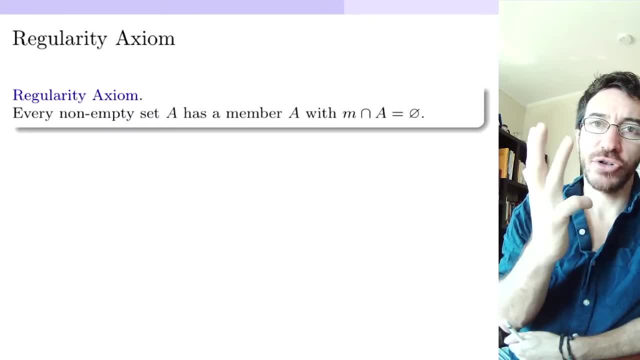 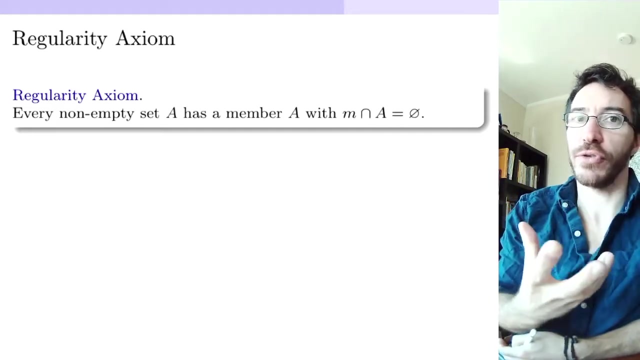 Extensionality, empty set, pairing, Union. those are the basic ones. then subset axiom, infinite set, axiom of choice, Replacement, and now we're gonna see regularity. and out of these axioms, Replacement and subset axiom were schemes. They were not a single axiom, but we had one for each sentence or one for each formula. 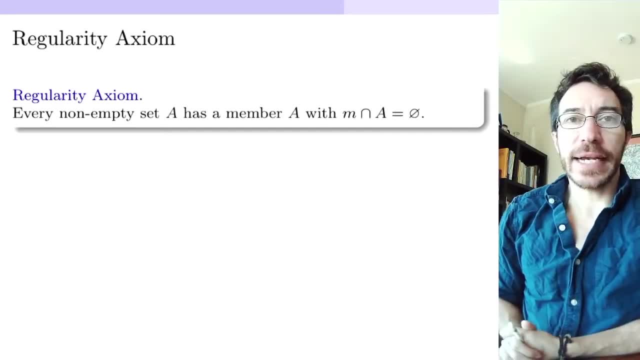 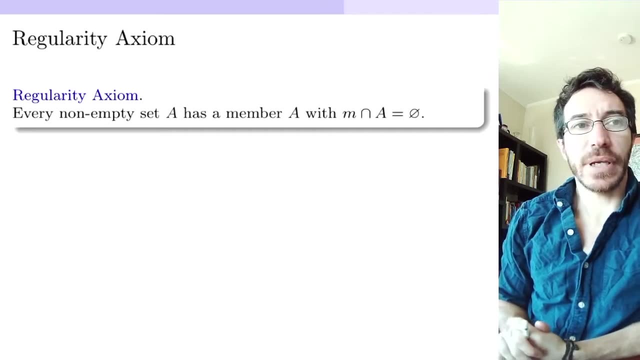 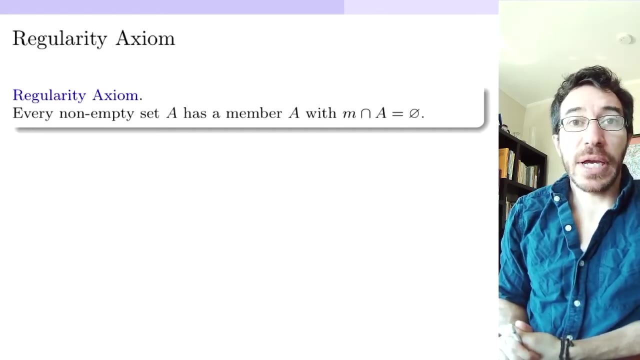 in those cases. Okay, so let's see what the regularity axiom says. This is kind of usually considered kind of the least important axiom, But makes things work nicely and, Yeah, it's well. it is always considered part of ZFZ. Yeah, we haven't used it so far, So I guess it gets more important later. 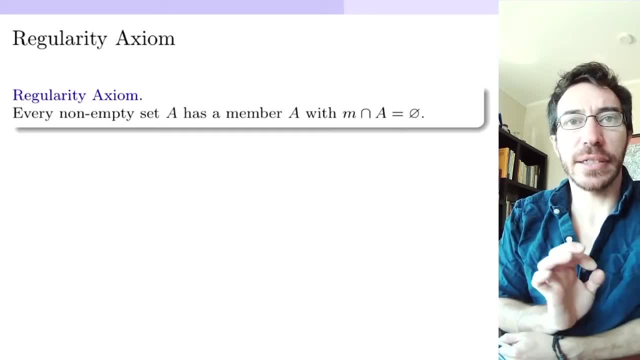 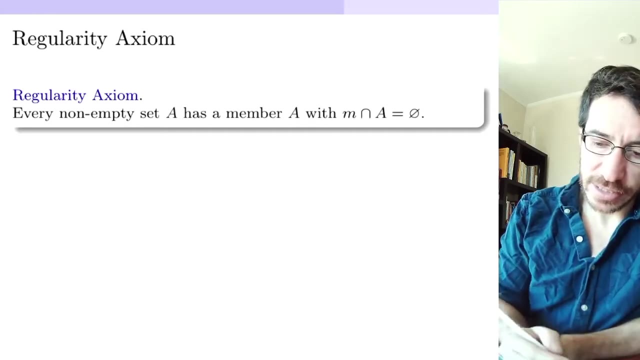 It's statement might look a bit obscure at first, but we'll analyze it And see what it means. So it says every non-empty set A has a member Which he has empty intersection with A, Okay so. So it's essentially saying: I'm gonna say it. in other words, 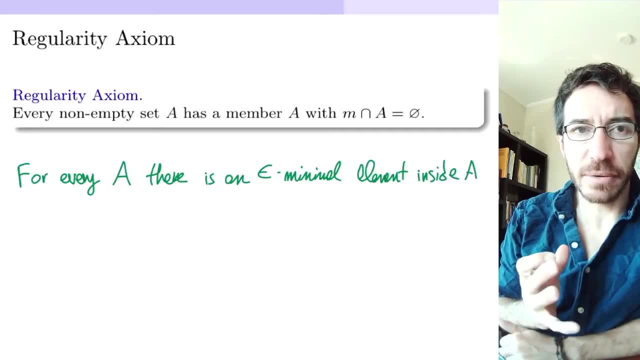 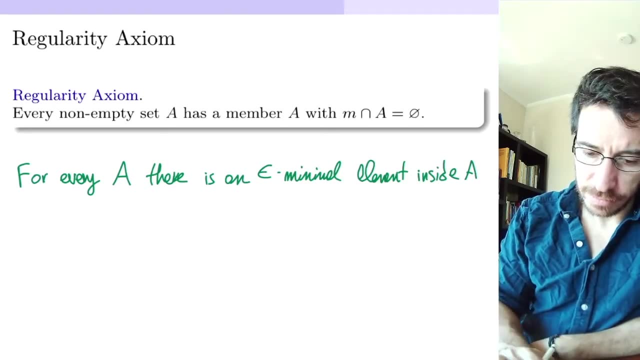 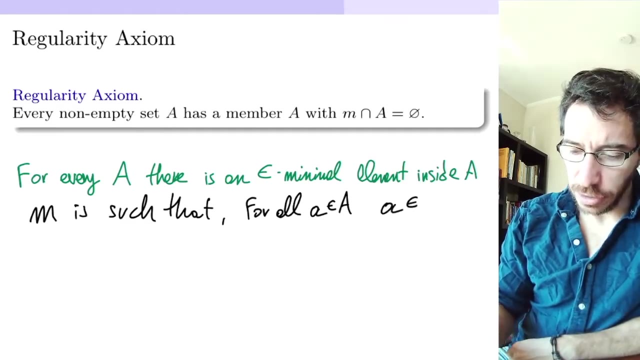 So just rewriting this says that for every set A there is an epsilon minimal element inside A. But epsilon minimal I mean, So let's call it M. This little, this minimal element M is such that for every other element in A, A does not belong to M. 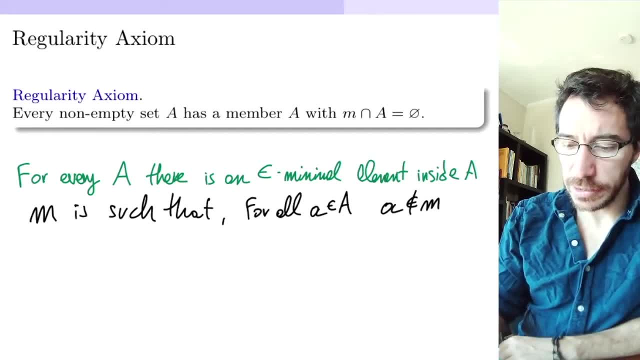 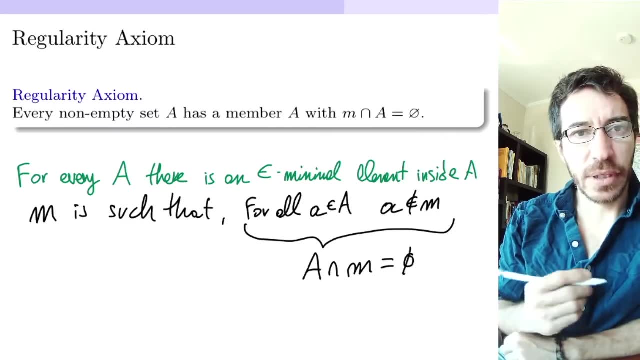 Okay, so that is the same thing. I mean, I'm just rewriting it. Essentially, this thing here is exactly the same as saying that A intersection M Is empty, but it's a different way to see. No, it's like among all the elements of A. 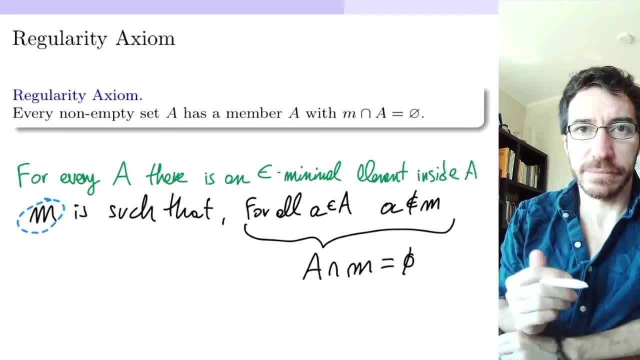 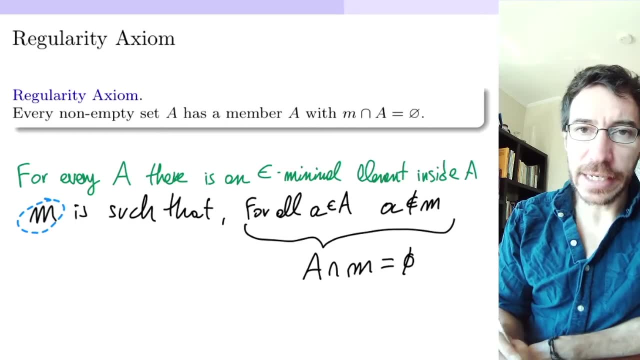 There is one, probably many, Maybe most or not, I don't know, but at least one Which Which doesn't contain any other member of A Right. So it's a least in terms of this relation. This is not an ordinary relation, actually It's not transitive. 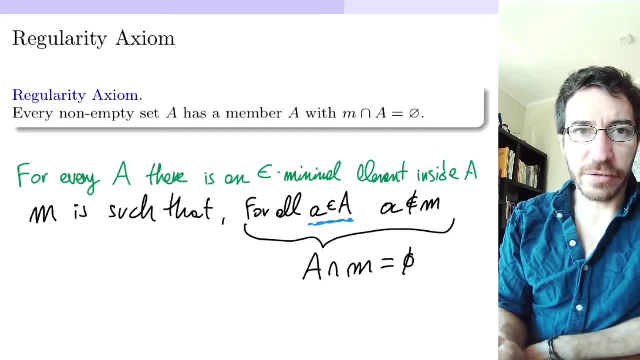 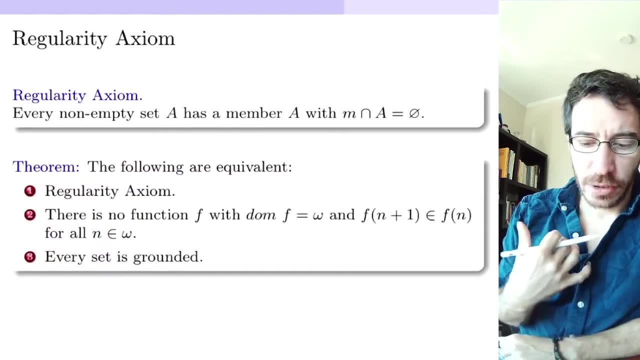 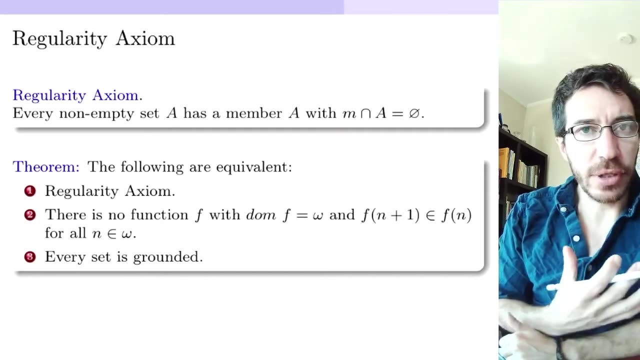 but it's least in that sense of for any other element of A little a is not in M right, That's what this says, So let's analyze it a bit further. This theorem is essentially the one that explicitly shows what it means. So these are three different. 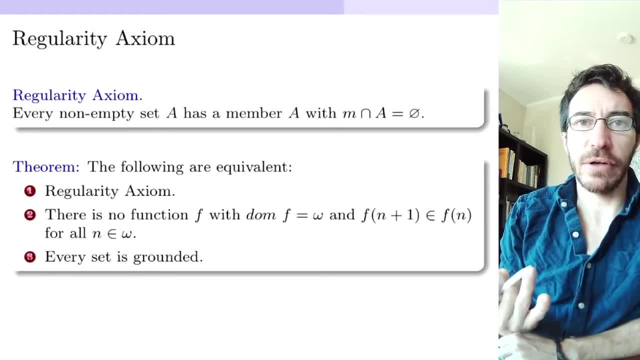 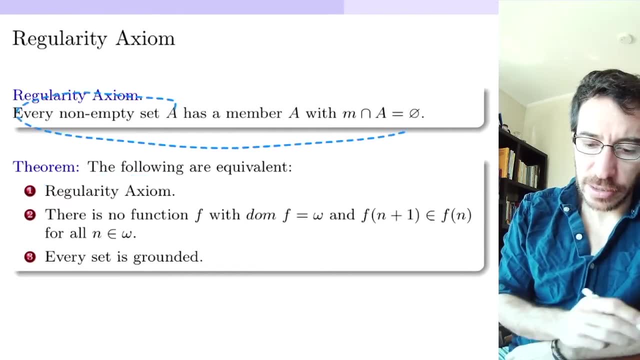 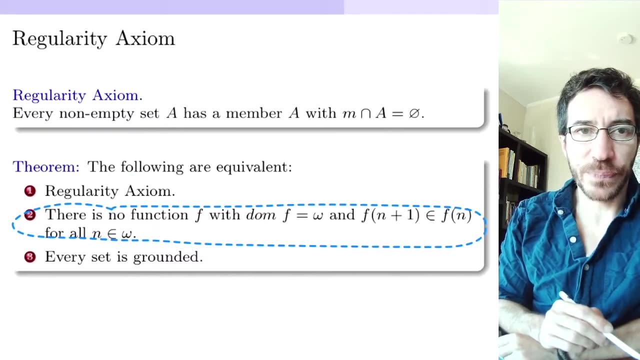 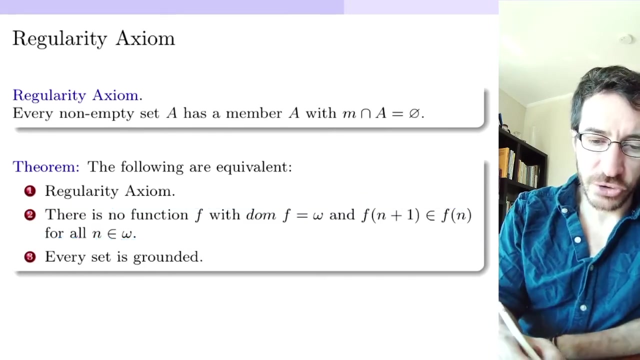 variations of the regularity axiom. These three statements are equivalent over the other axioms of CFC, and so one is the regularity axiom that we just stated. Then this one: there is no function With domain-denatural numbers, such that f belongs to f for all n. So in other words, this is saying no. 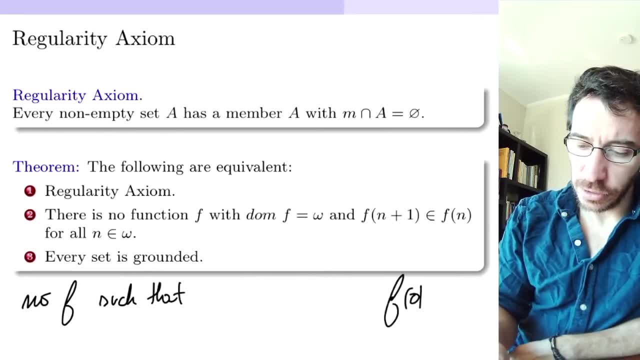 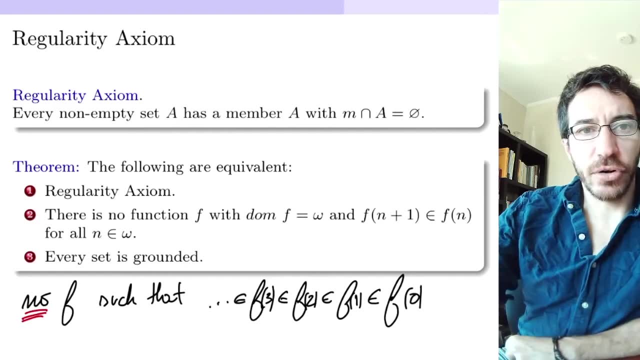 function f such that f contains f. Right, that's what number two is saying. There is no descending sequence like that. On, like, on the belong relation, you're gonna have something that belongs to something, that belongs to something, And all the way down in that direction. 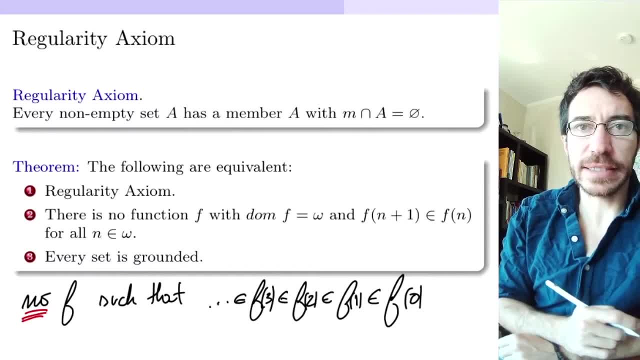 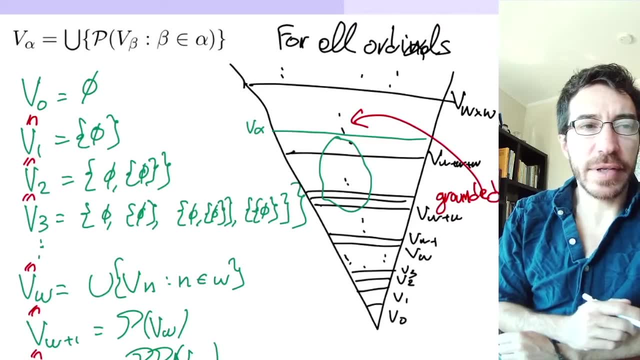 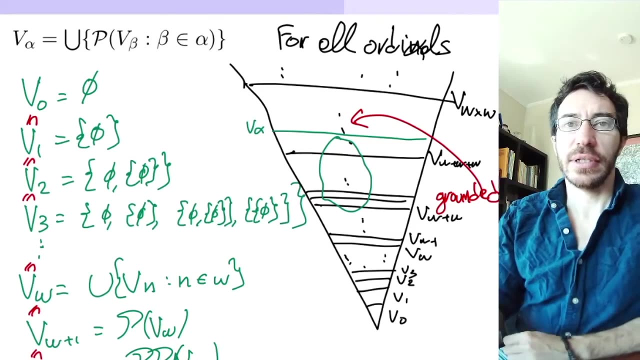 And number three, it says that every set is grounded. You guys remember what that is. That's from the last video that we did last week. Remember the definition of the V hierarchy, Where it's a hierarchy defined on all ordinals, not just up to an ordinal? Last week we saw how to define it on all ordinals. 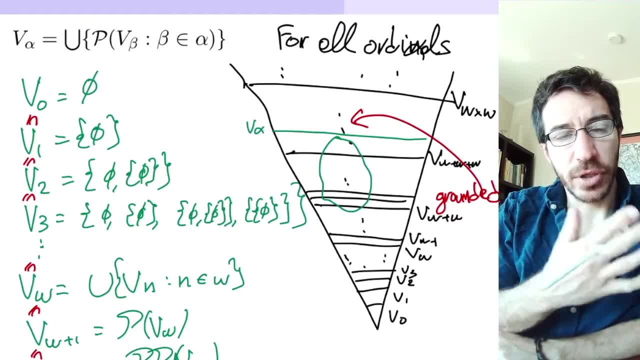 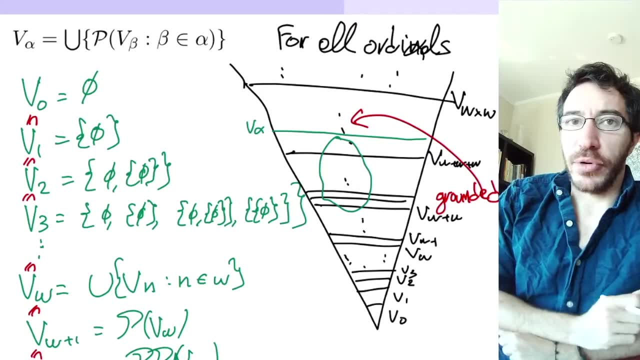 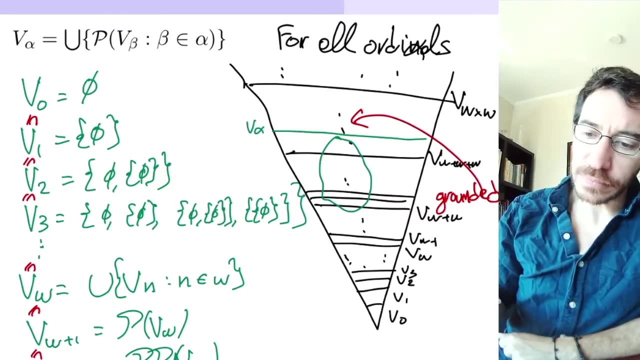 and the idea is that each one is the power set of the previous ones, Because we start with the empty set. they are all containing charges And there is a sequence growing and growing and growing of of more and more and more sets, and It go grows all the way through all the ordinals. 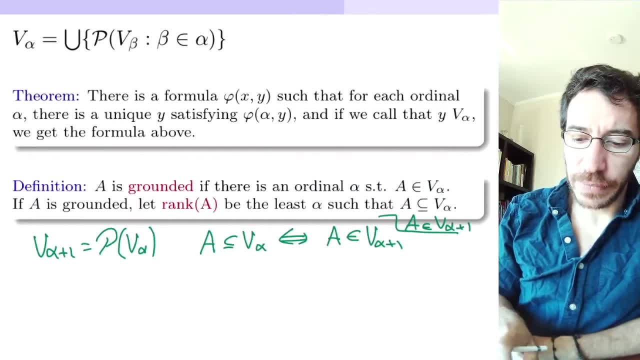 And then we define a set to be grounded. If it belongs to one of these V alphas, are equivalent. is a subset of one of these V alphas, the same thing is belonging to the next one. essentially, So that's what he meant for a set to be grounded. 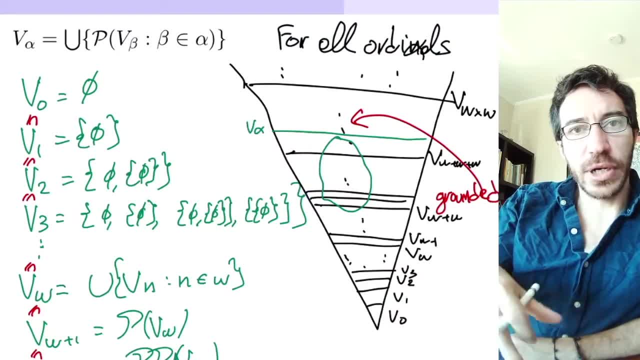 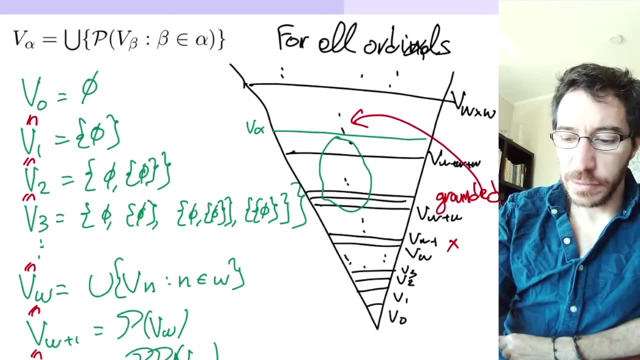 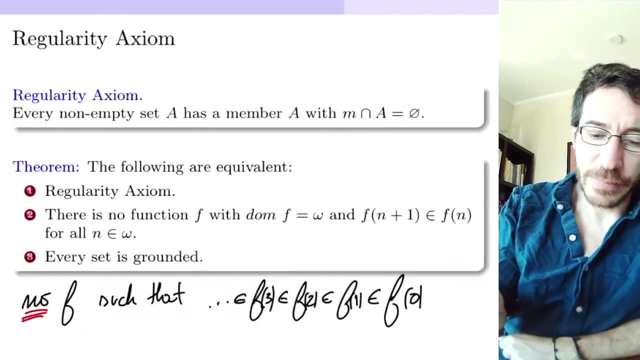 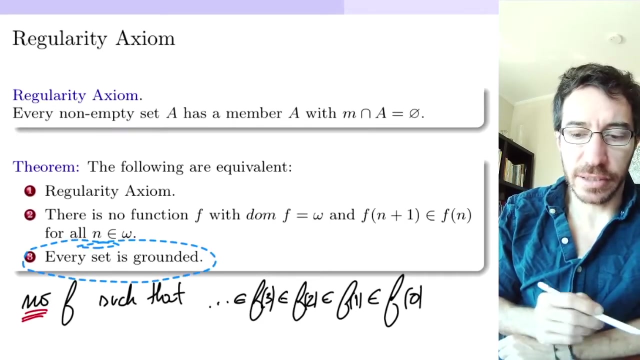 that it belongs somewhere in this v-shaped hierarchy. So a non-grounded element will be up here. this will be not An element outside that hierarchy. that is never built using this power set. What regularity axiom the third equivalent says is: every set is ground. So it says for every set A, there exist alpha and ordinal. 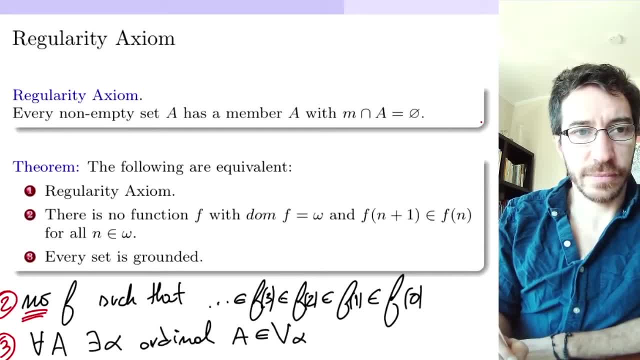 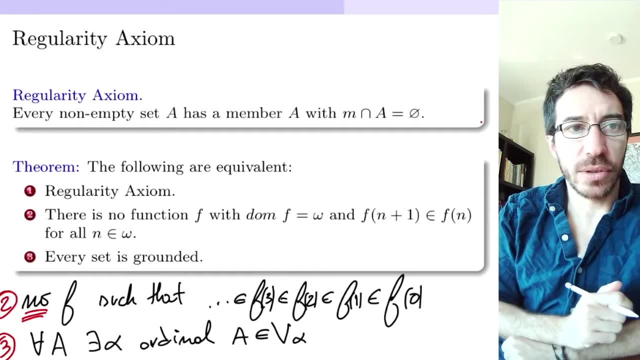 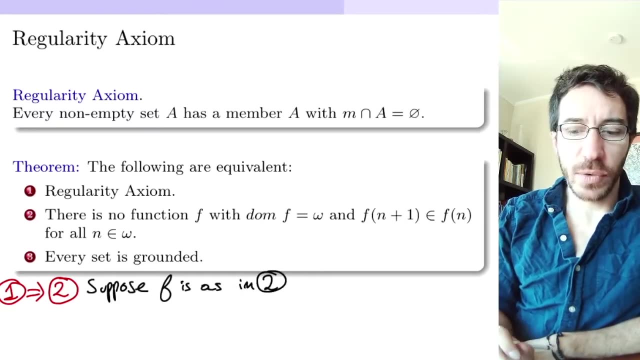 such that A belongs to V alpha. That's what number three says. Okay, so let's prove these three are equivalent. To prove that one implies two, let's do it by contradiction. Suppose there is such a function, And then what do we do? 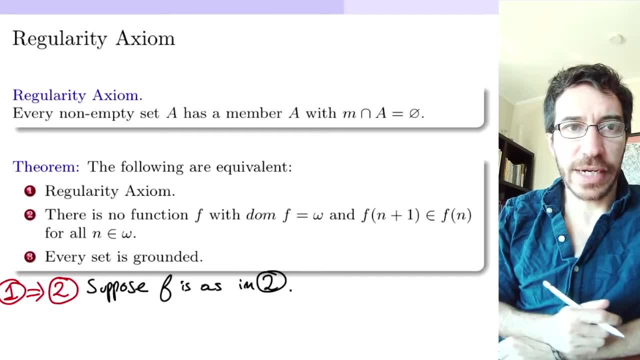 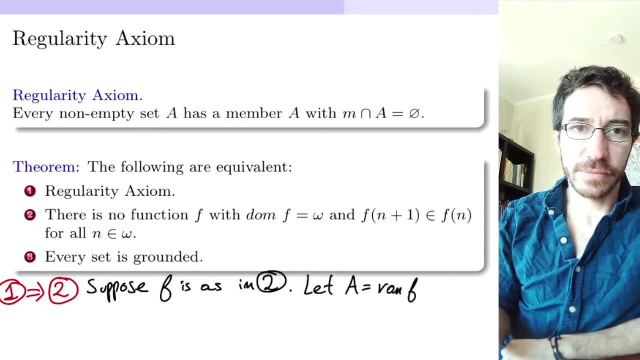 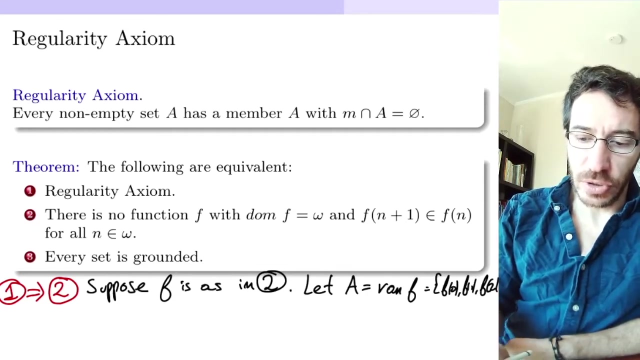 Well, we want to contradict number one. So we want to find a set A that has no belongs list element. What is that going to be? Well, the range of f, namely the set f0, f1,, f2, f3, f4, all the way, all of those guys. So is that what we want? 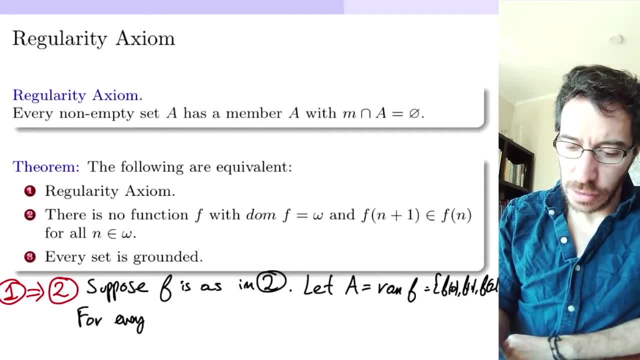 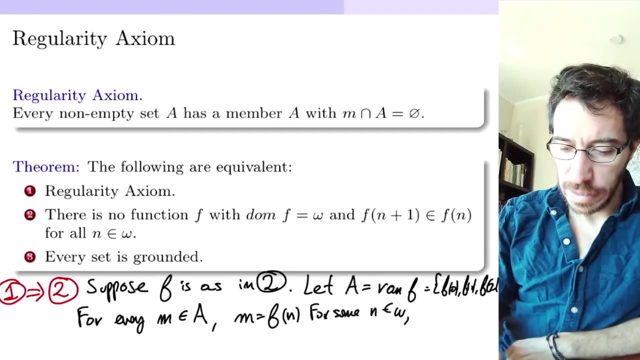 Right, yeah, So then this has no list element, right? So for every m that belongs to A, say m equals a to n, for some n in the natural numbers and f, n plus one belongs to m and belongs to A. 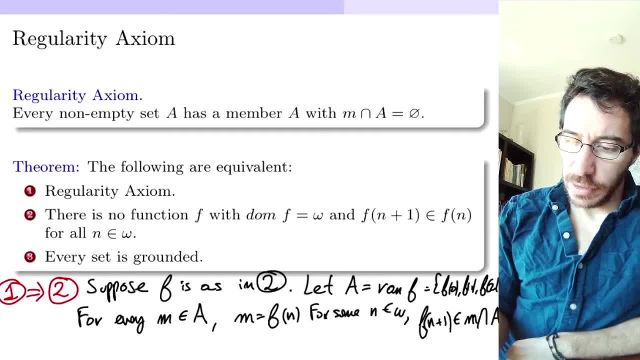 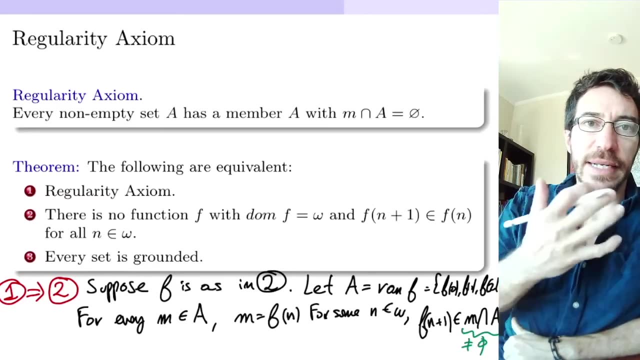 Right, contradicting the regularity axiom, that there has to be some m, such that the intersection is empty. right, So we get that this is for every m. this is not empty, And the regularity axiom says that there has to be some. that is a list, right? So there is no list in this case. Okay, so that proves one implies: 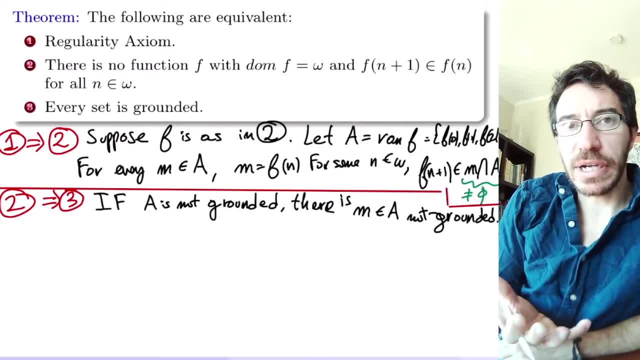 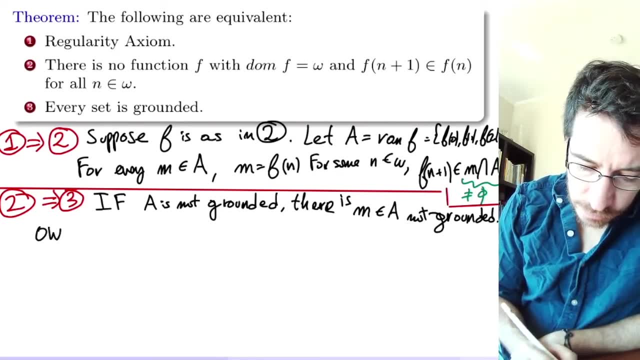 two, If A is not grounded, whenever you have a set that is not grounded, there must be an element inside which is also not grounded. Why is that? Because otherwise, if we let alpha be the supremum of the ranks of m. 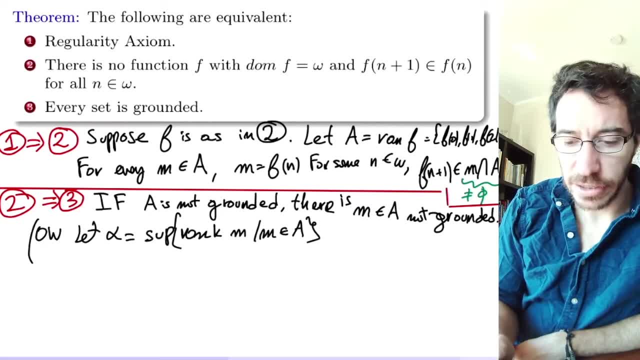 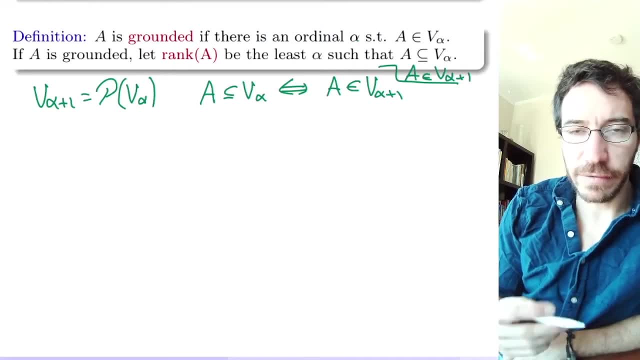 for m in A. remember that if a set is grounded then all its elements have a rank. Well, it has a rank which is the least alpha, that belongs to v alpha, but it's a subset of v alpha, so it belongs to v alpha plus one, right? So if we define, actually let's put rank of m plus one. 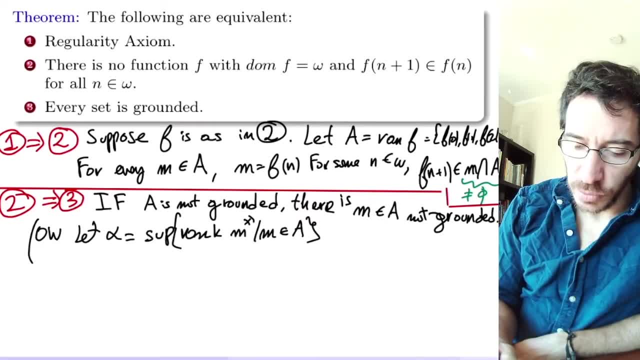 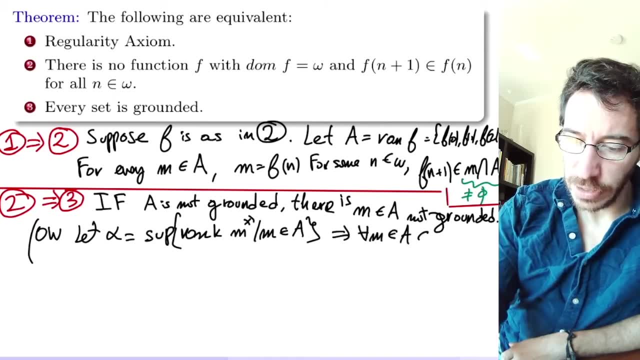 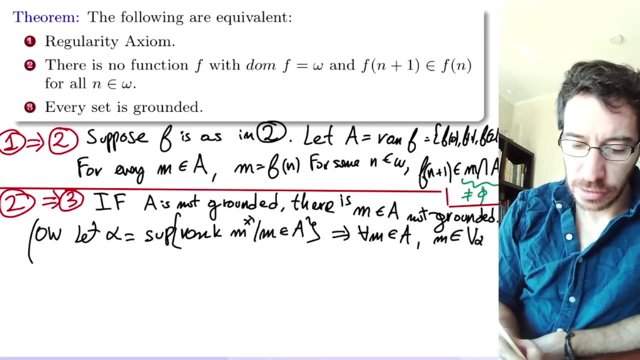 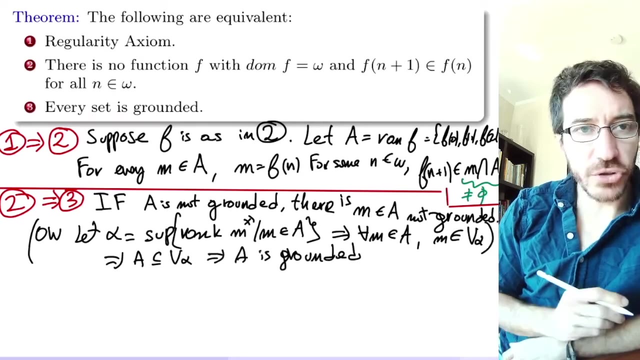 the supremum of all these guys, for n in A. so then you will get that every m in A, for every m in A, m belongs to v alpha, because we put the rank plus one, but then we get that A is a subset of v alpha and therefore A is grounded right. So 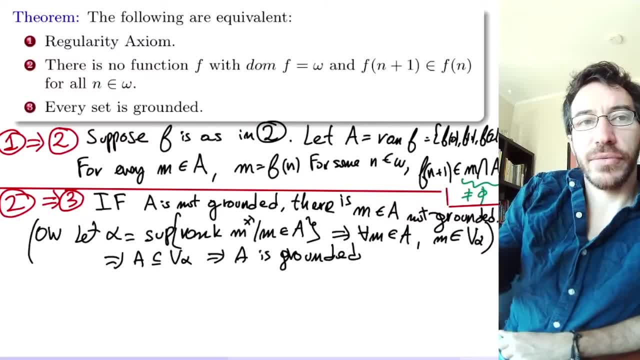 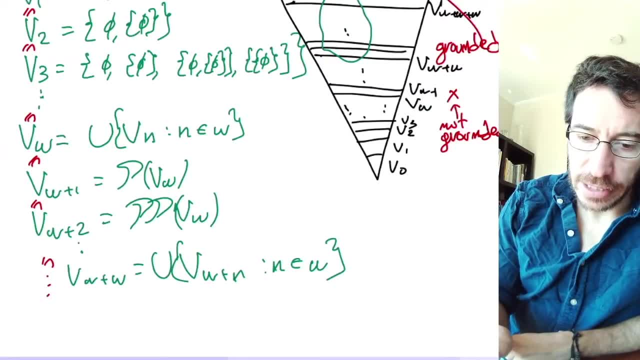 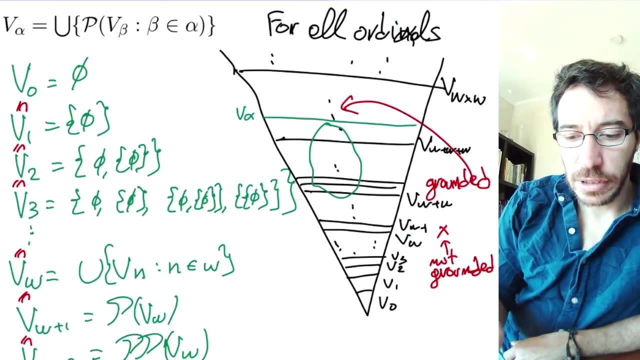 if all your elements are grounded, they all belong to some v alpha. this is the supremum of all the ranks, of all the elements, like in the picture right here. if you have these green sets right here, all the elements have some rank in here. if you take the supremum of all these elements, of all these ranks, 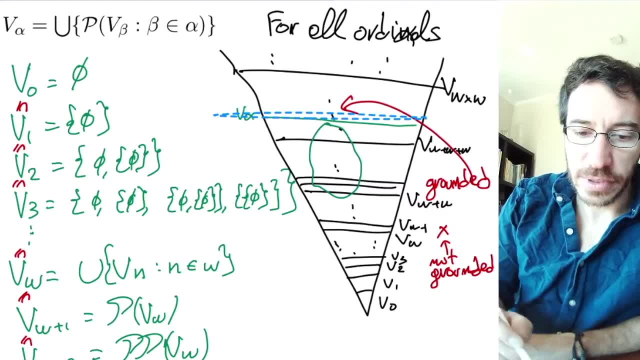 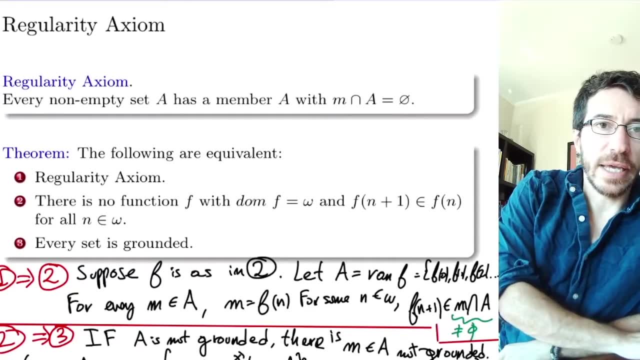 you get this v alpha and then A belongs to subset of v alpha. Okay, so if all the elements inside are grounded, then A has to be grounded. so the other way around: if A is not grounded, then one of its elements must be non-grounded. so let's so. the idea for the proof is now to build a descending 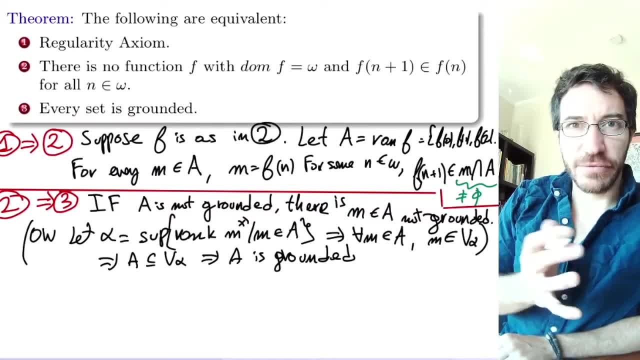 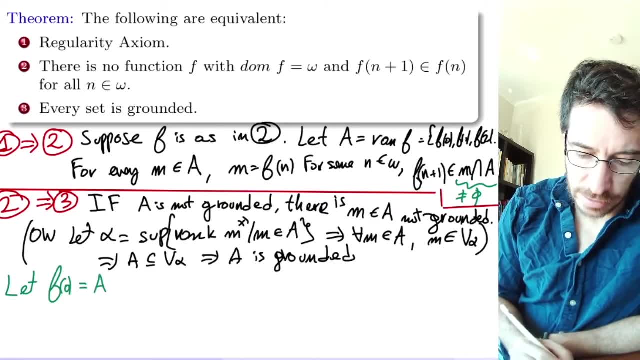 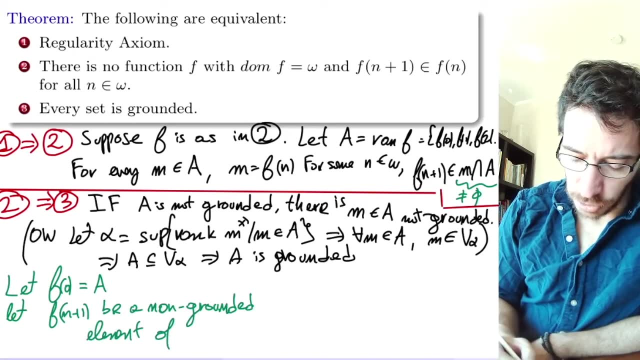 sequence of non-grounded elements going down. So let's first define it and then fix the details. So let f of zero be A and let f n plus one be a member, a non-grounded element of f of n, so we manage. so the idea is we define the sequence at every time we choose elements. 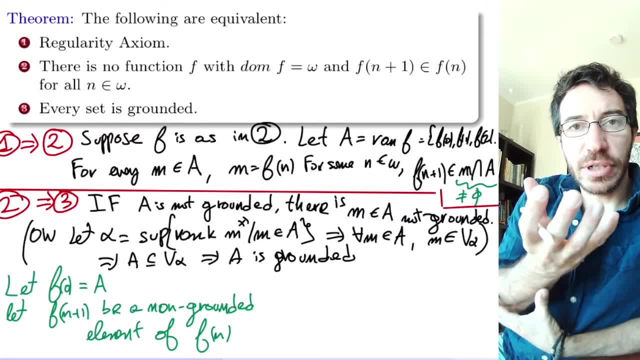 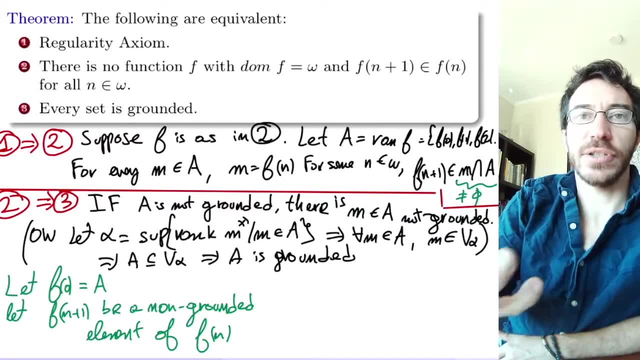 that are non-grounded, and every element that is non-grounded has an element inside that is non-grounded. So that's our next f, And since that one is non-grounded, it has an element inside that is non-grounded, We choose that one. 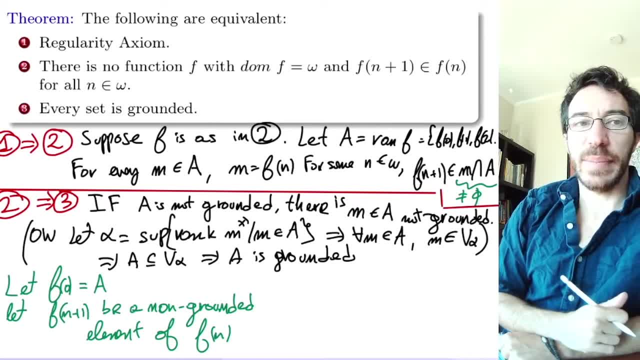 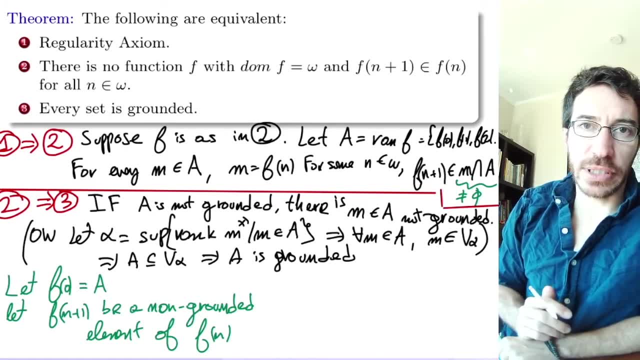 And we keep on going like that, always choosing an element inside non-grounded. There's an obvious use of the action of choice here, because you have to choose one of these non-grounded elements. So if you want to be careful of where we're, 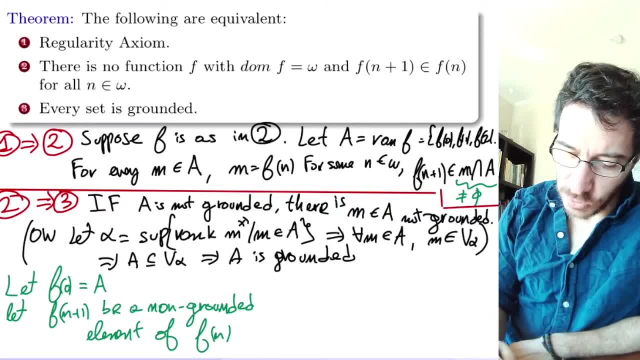 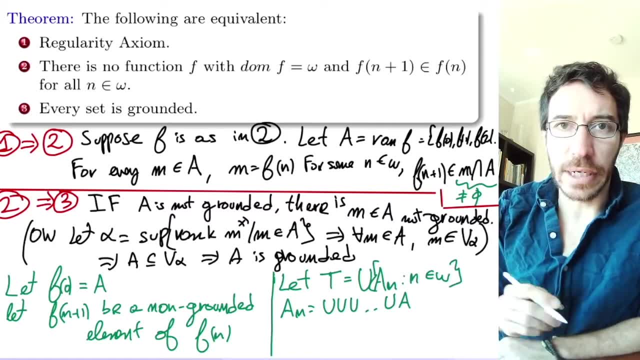 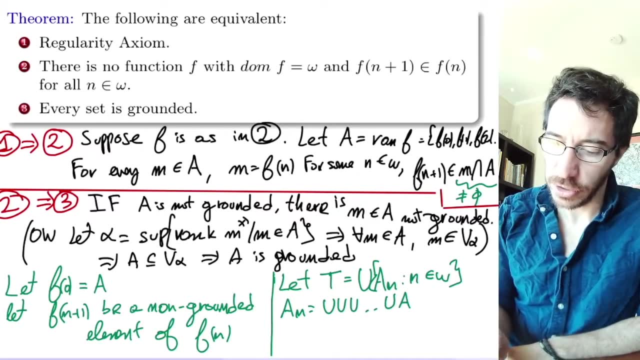 choosing these guys. we have to do just a little trick: Okay, to apply the action of choice carefully. we need to do this little trick. We know how to define T with the transitive closure of the sets of A, which I guess you did in the. 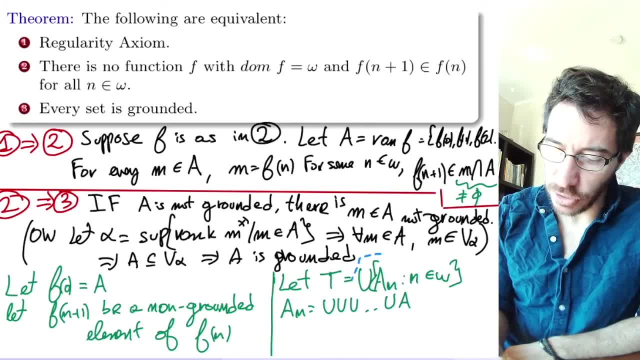 homework. So this T is the union of all these guys, A sub n, where A sub n is the union of the union, of the union of A? n times. So what is the union of the union of A n times is all the elements that belong to. 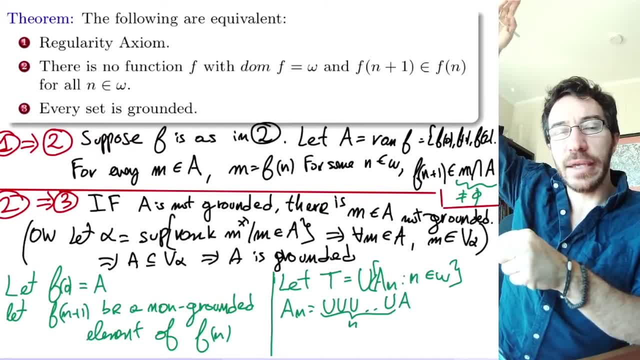 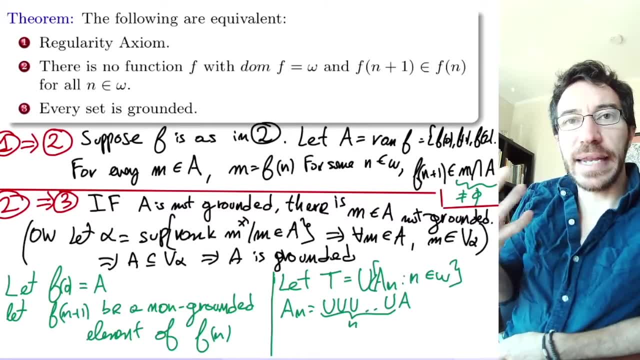 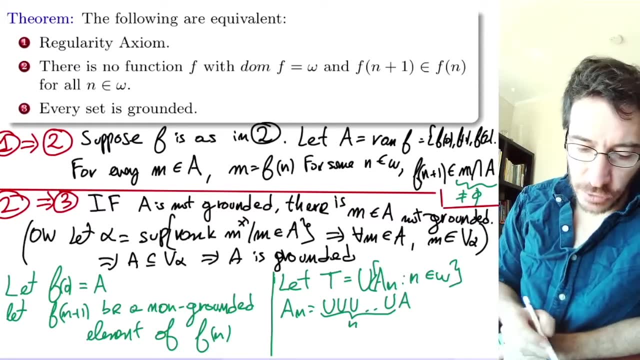 something that belongs to something. that belongs to something that belongs to A or that n belongs to in the chain of length N and the union is for all n's. So we are taking anything that belongs to something belongs to something any number of times until you reach A. and if you see these functions, 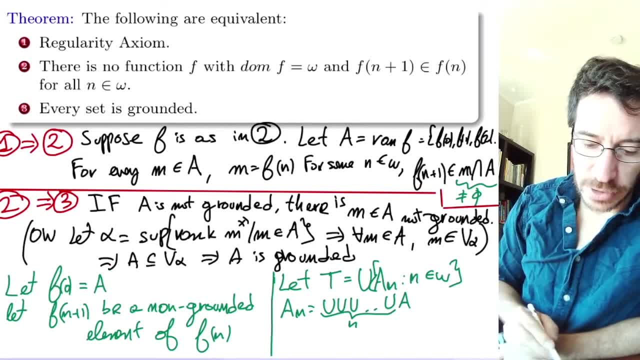 we are defining. very here they are of that, We start with something in A and then we take something that belongs to A and then we take the other wood. We saved the choosing to At a. we went back to at A and 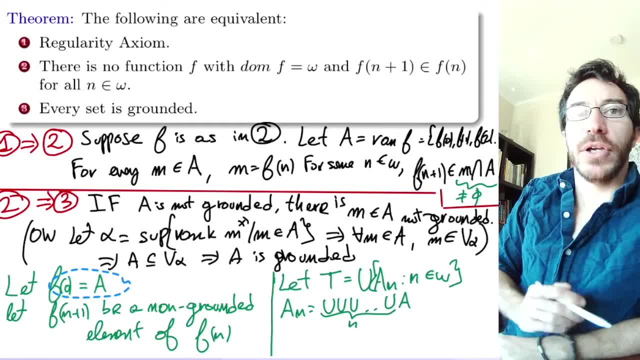 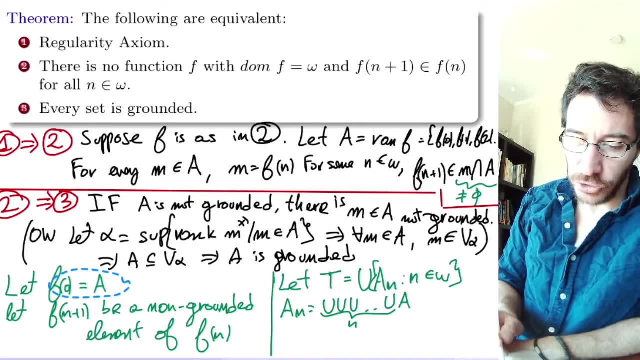 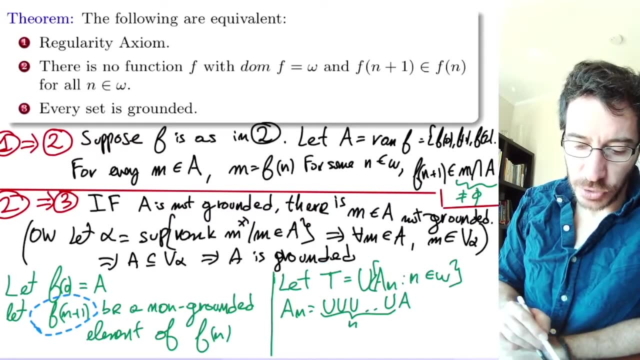 something that belongs to that and something that belongs to that. okay, So now, if we use the axiom of choice on the subset of T, and for each subset of T we can choose an element, these Fs- Ns are always choosing here. they're always choosing in between the non-grounded 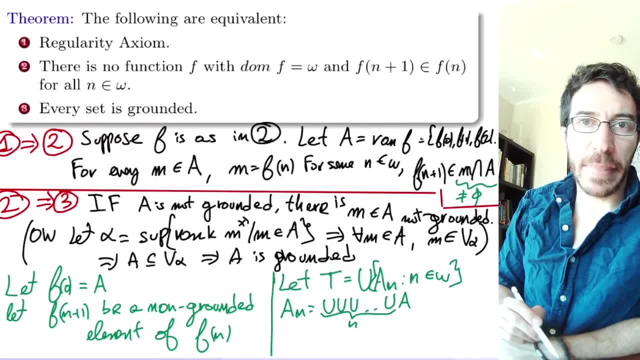 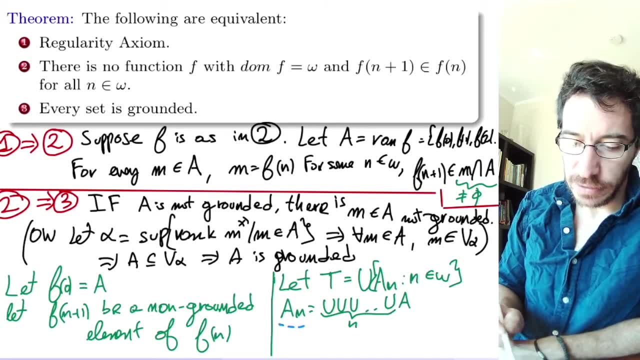 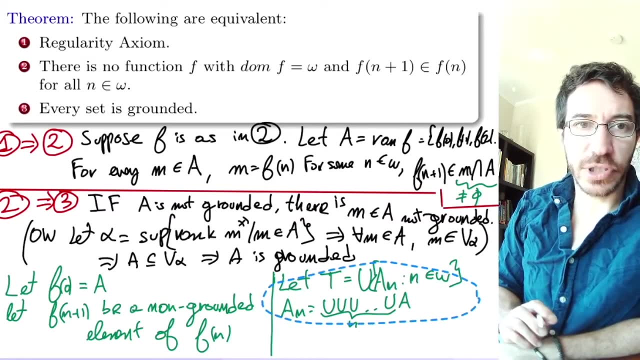 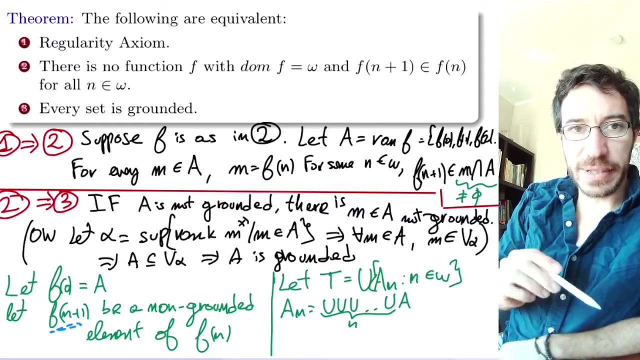 elements of F sub N, which is a member of, which is a subset of T right, Or a subset of essentially, a N, if you want. Okay, so the axiom of choice can be used correctly if you consider this transitive closure, but essentially what we're doing is that just picking, choosing an element that belongs to. 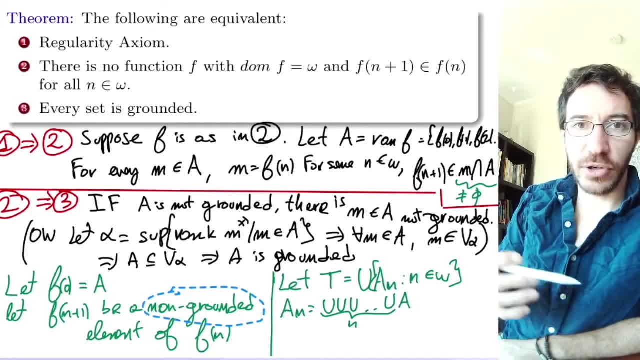 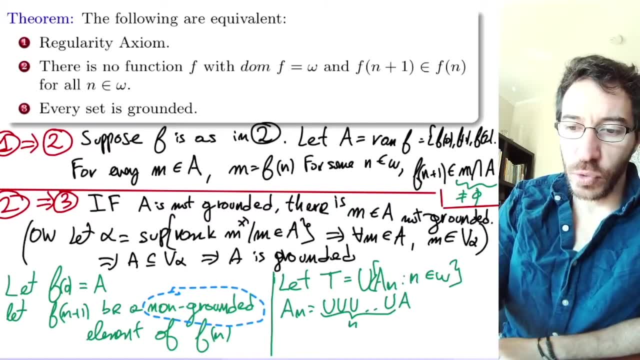 the previous one, making sure that it's always non-grounded, so you can always choose a new one, because every non-grounded set has a non-grounded element. Cool. so that's the proof that 2 implies 3, less non-grounded. 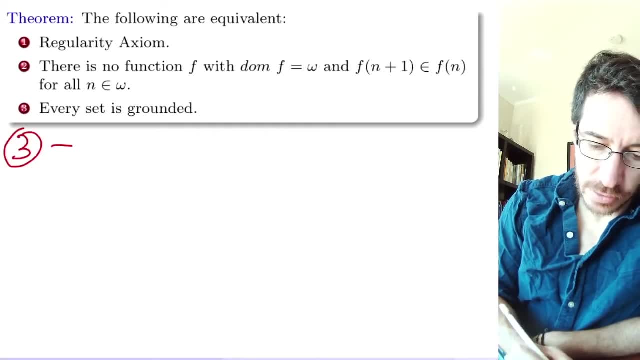 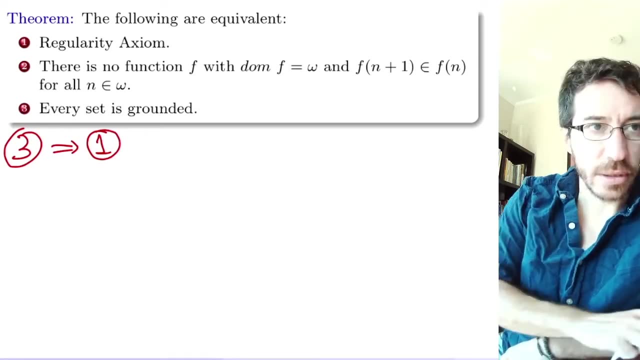 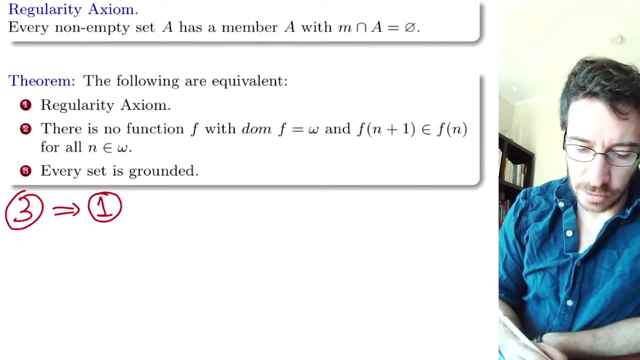 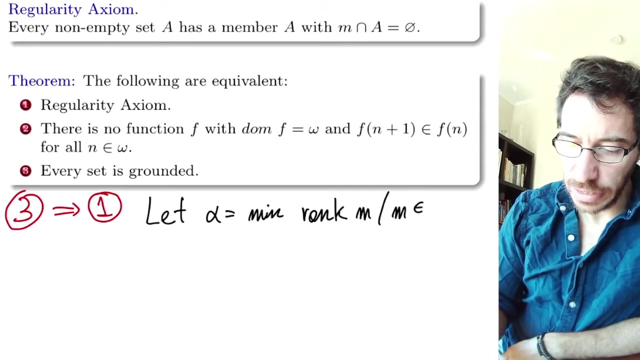 Let's now prove that 3 implies 1, okay, So now we're assuming every set is grounded. let's put the replacement axiom back in so you can see what it says. So we have to take a set A. now let alpha be the minimum of the ranks of M, for M that belongs to A. 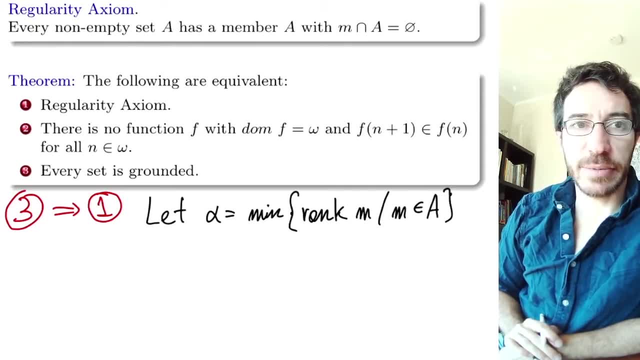 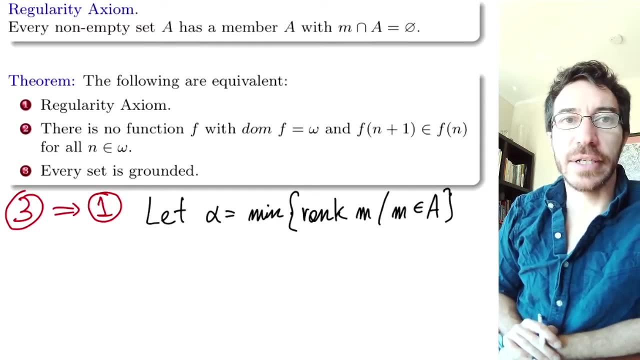 right. If every set is grounded, every set has a rank. that's the assumption. That's the assumption That every set has a rank. A rank is the first alpha set that you belong to V of and you're a subset of V of. So, among all the elements of A, you'll have a rank. 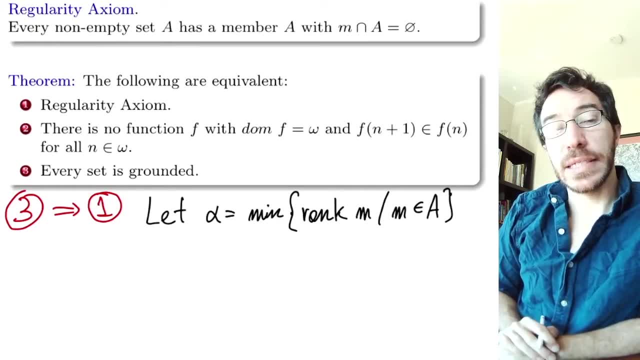 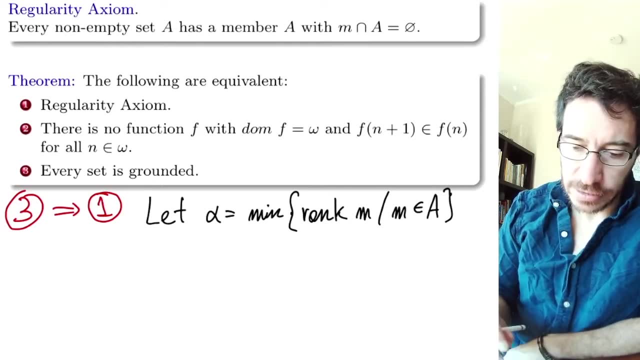 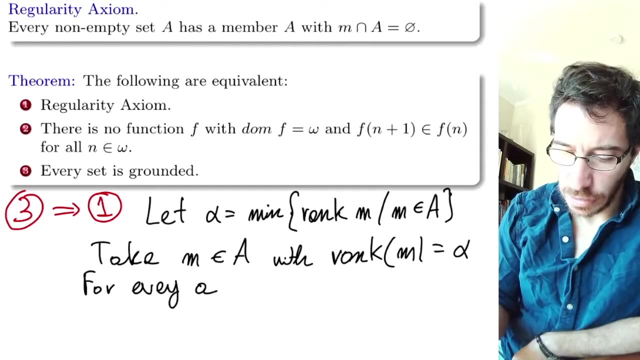 so by replacement, this set exists. This is a set of ordinals, so it has to have a list element, because every set of ordinals has a list element. so that's the alpha. and now take M in A with minimal rank. okay, Now for every A in A, we have that. 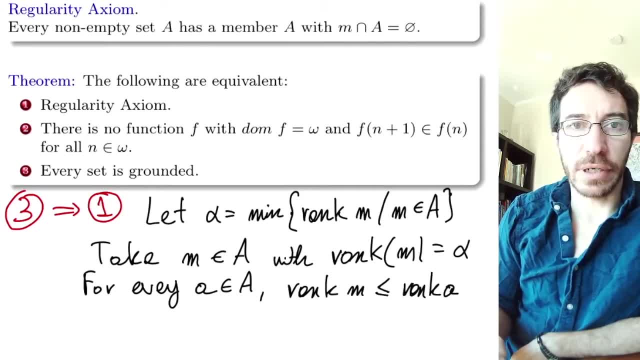 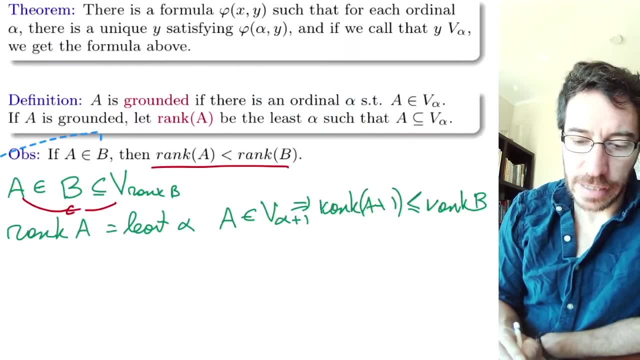 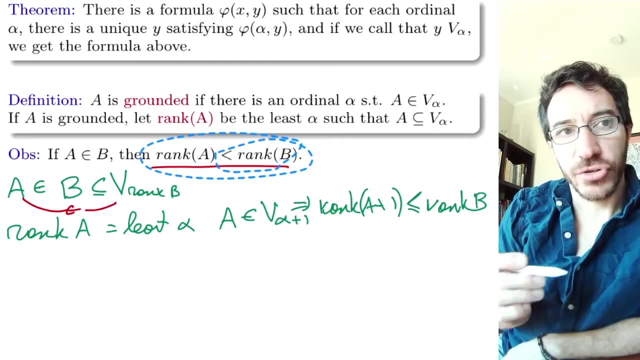 the rank of M is less than or equal the rank of A. And if you remember from last time, we showed that, this observation that if A as a set belongs to another, then the rank has to be strictly below the other right. So in this case, 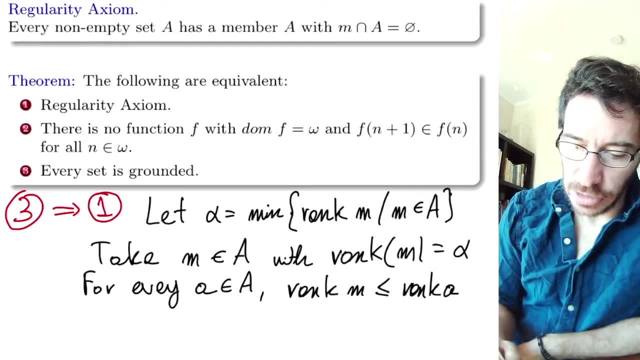 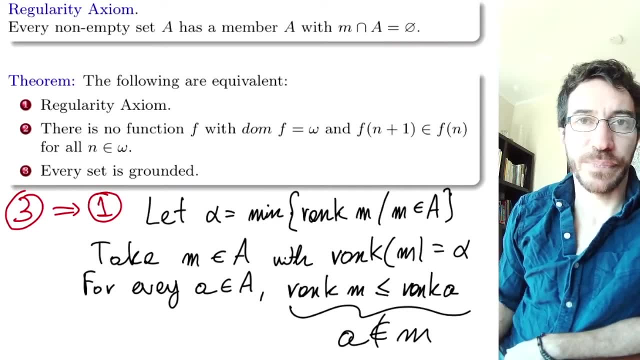 the rank is not strictly below. so this here implies that A does not belong to M, so M is a minimum element. Okay, So that's the assumption. So now we're assuming every set belongs to A and we're going to take M as the set of ordinals. Okay, So that finishes the proof of these three. 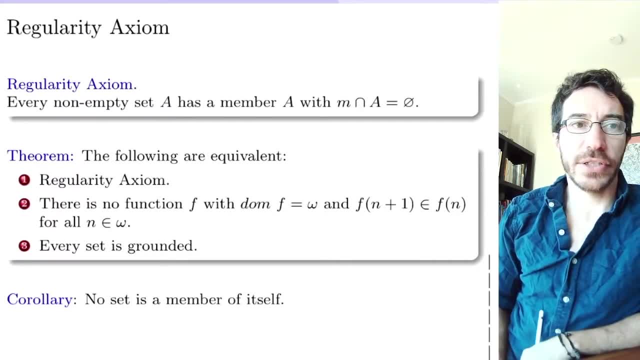 equivalents. One corollary of this regularity axiom, of this theorem, I guess, is that no set is a member of itself. Remember, we mentioned this at the very beginning. we asked this question and kind of analyzed it intuitively. It follows from the regularity axiom right. 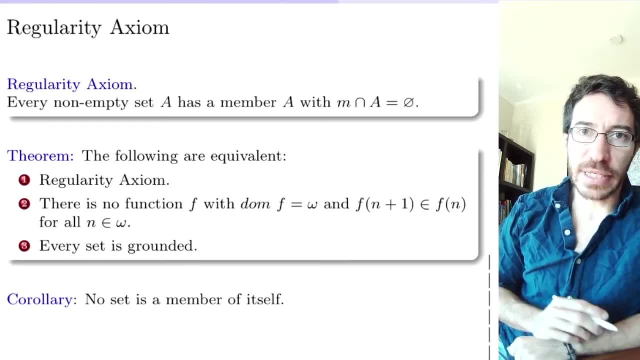 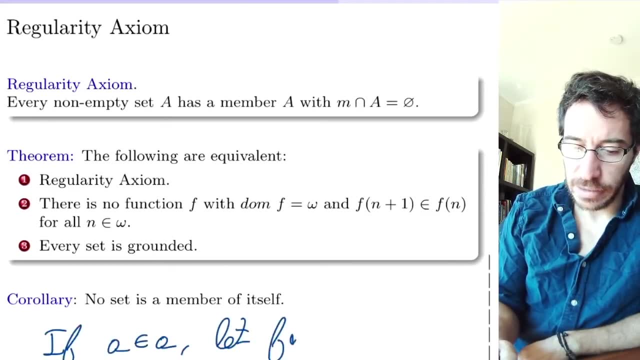 Because you cannot have. if you had a set that belongs to itself, then you define M as F. So if A belongs to A, you find, let F of N be A for all, A for all Ns, and then you get a. 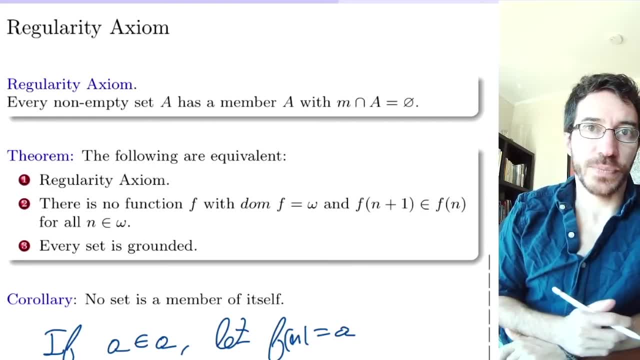 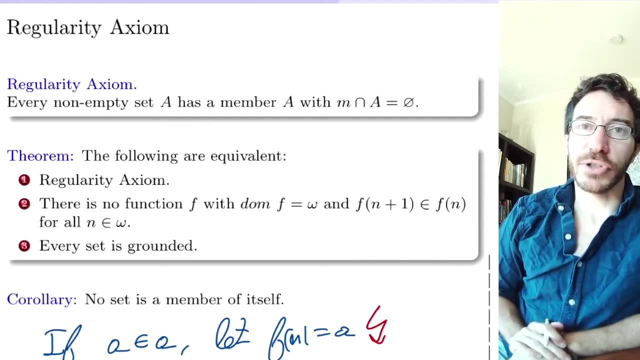 sequence that contradicts 2.. So you couldn't have that. So no set belongs to itself, And that simplifies also our lives a little bit so we don't have to worry about strange cases. So we had proved before that no ordinal belongs to itself, because ordinal is a 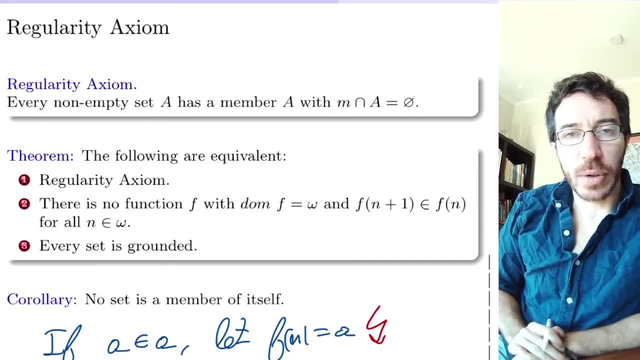 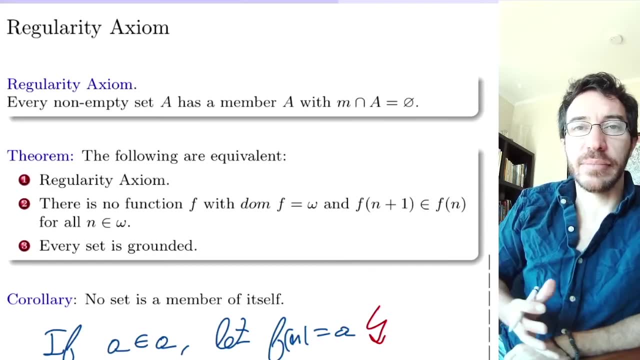 particular kind of sets And for those we could prove this without using the regularity axiom. In general you need to use regularity axiom. I guess it's easy to show that no grounded set belongs to itself because of the rank. They have to have a rank. But since now 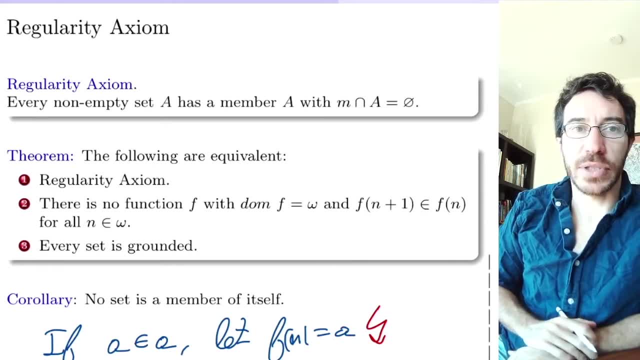 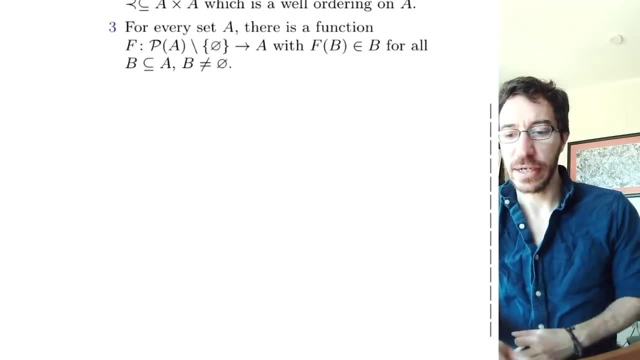 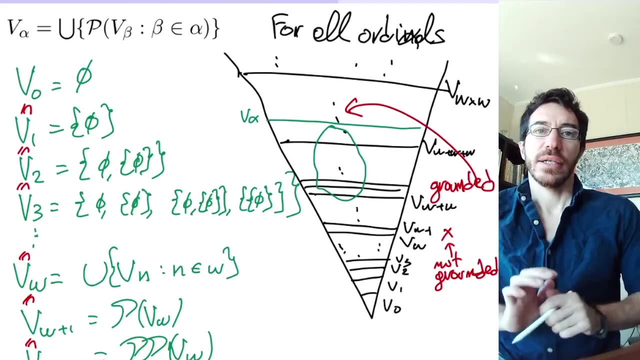 since regularity says that every set is grounded. no set can belong to itself. So the regularity axiom, essentially, is telling you this: It's telling you that this V hierarchy holds all the sets belong to this V hierarchy. And now we have a good picture of what our universe 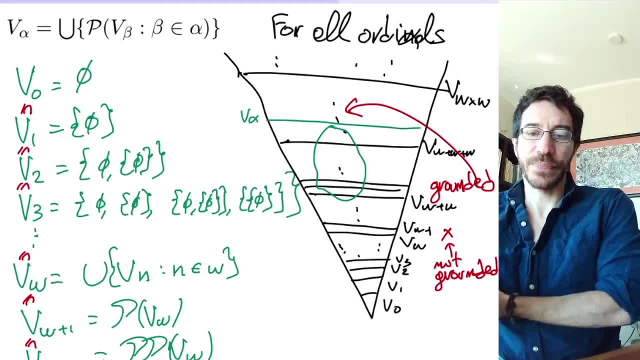 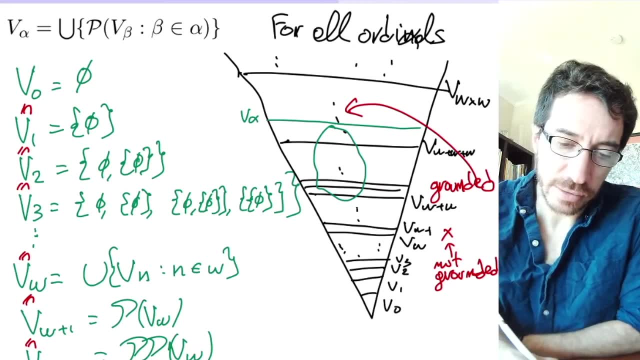 of sets looks like. Inside this universe of sets there are the ordinals And ordinals. usually they are depicted like this In V0, there is one ordinal, but this is nothing Here. this guy here is zero, And here you have one and zero, Here you have.